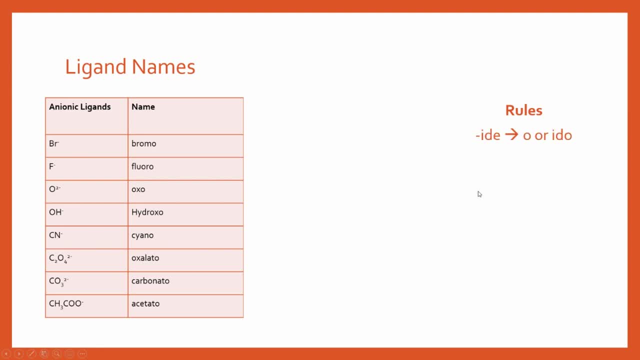 is a general rule for figuring these out. So the rules are that ide either becomes o or ido, and these can be used interchangeably. Typically, most of the time, you'll see names where the ide has become o, but also more modern texts sometimes use ido. 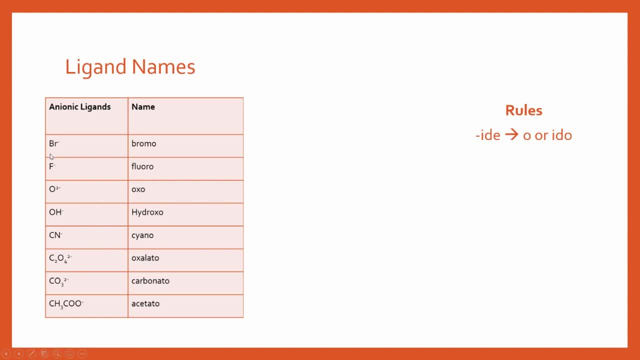 So you can see both of these being used. So, for example, this would be the bromide ion and that's becoming bromo. This would be the fluoride ion that's becoming fluoro, and so on. So you've also got another rule where et becomes eto. So, for example, this would be carbonate and it's become. 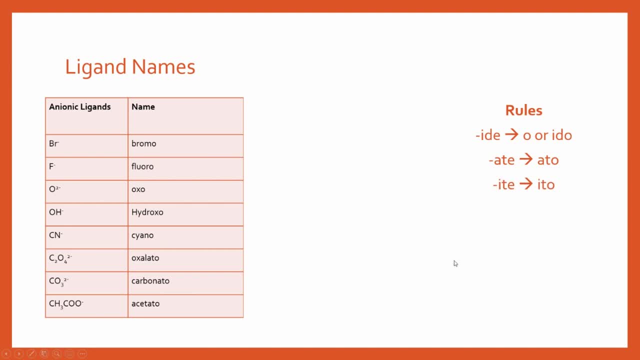 carbonato, And so that's how that's changed. Infrequently you might see ite and that would change to ito, And then we also have other possibilities. So, for example, if you have a neutral ligand, you might have a neutral ligand. So you may have neutral ligands and these have got. 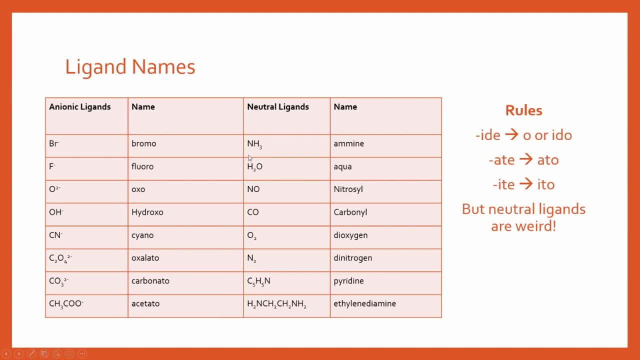 weird names. There's not a simple rule like that. So, for example, for a neutral ligand, you might have NH3. That would be called an amine in the name, H2O would be aqua, And then so on. We've got all. 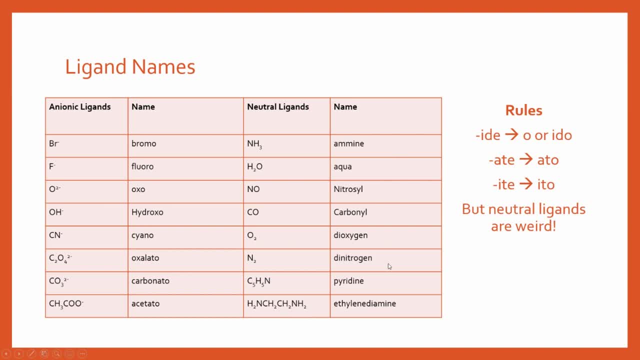 these other names, One of the ones that's going to be useful in this video- we don't use all of these, but these are common ones- is this complicated one down at the bottom? This is your ethylene dye amine and that is going to be a bidentate ligand. 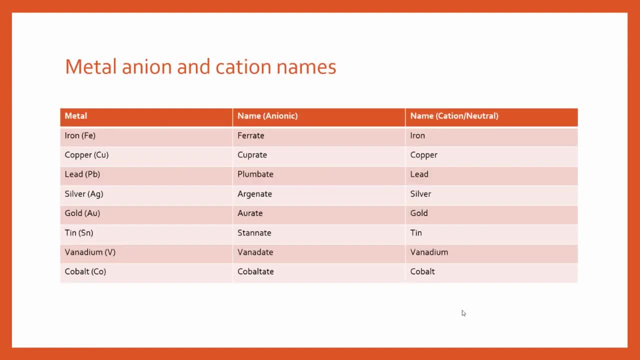 It's going to be important a little bit later. So that's one of the key ideas. The second one, and it looks like there's a lot of information here, but it's all the same thing really when you look at it. So you've got anions, cations or neutrals, and it depends what charge is present as to what you're. 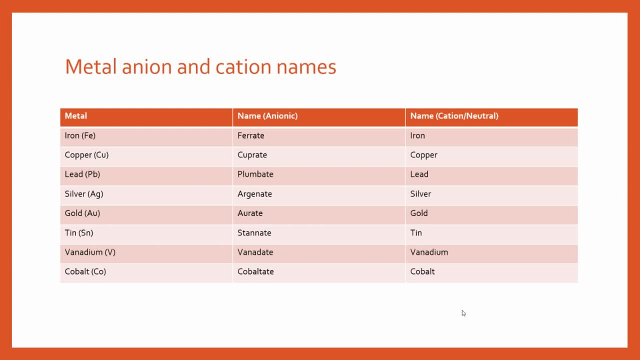 going to name the metal in the name of the coordination complex- coordination compound or the complex ion. So if you had iron, for example, we would be calling it ferrate in ionic conditions or just iron if it was a cation or neutral. And likewise copper would be cuprate. 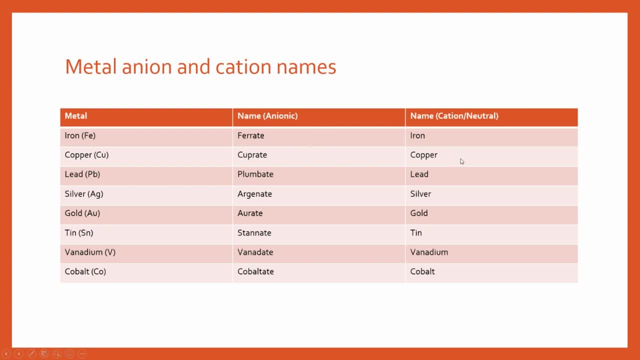 in ionic conditions and copper, if it was to be a cation or neutral. And you'll notice that these are generally coming from Latin and so you might recognize the Latin names here. And that's how you're going to come up with these names. You have to figure out whether you've got an anion. 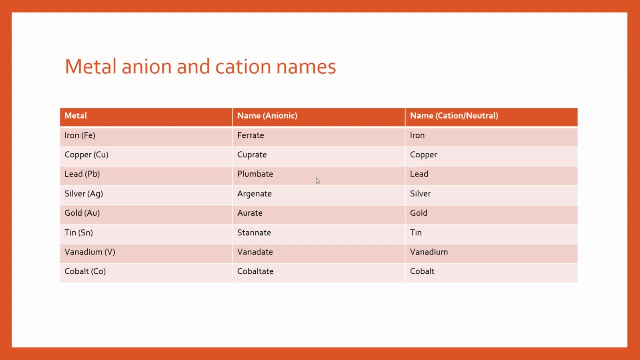 or a cation, or a neutral substance, and then you can work out which one of these to use. Now I'll put on the bottom of each of my examples extracts from this table, so you don't have to memorize all of them. So let's move on and look. 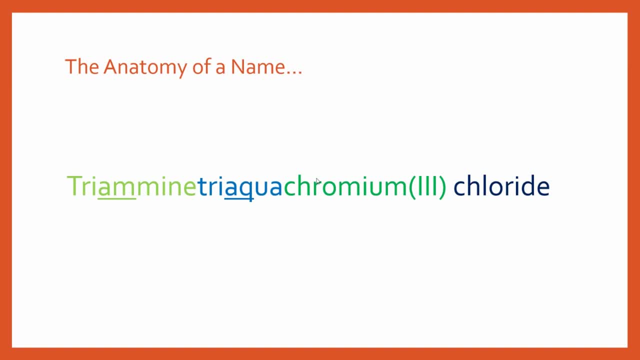 at the actual anatomy of a name. So here is just the name that I've picked out, and what we have is some underlying things, and this is one thing I want to highlight. We've got am for amine and aq at the start of aqua, and these are the ligands that are going to be present in this substance. 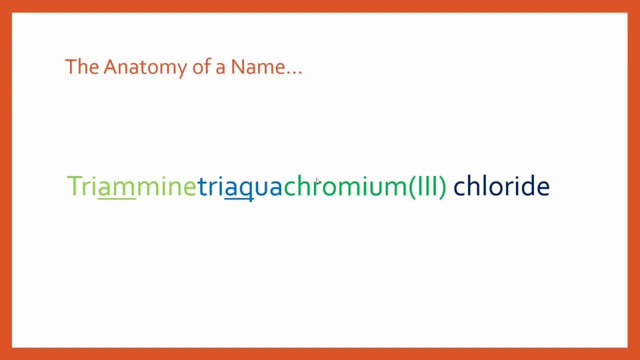 The key thing to notice is that they go in alphabetical order. so make sure you put your ligands in alphabetical order, otherwise it's wrong. So let's look at this name and break it down. So the triamine means that we've got three NH3s. The triaqua means we've got three H2Os. 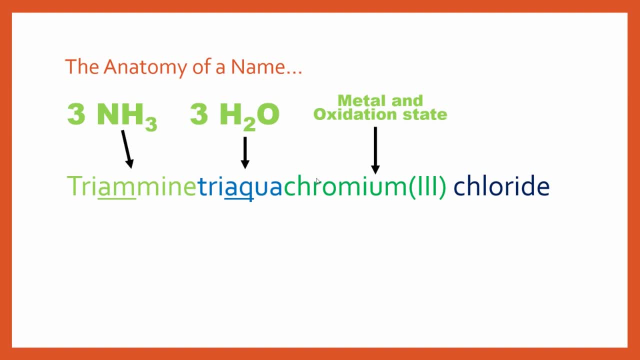 The chromium, with the three, is the metal in the oxidation state, and then the chlorine is sometimes called the counter ion. So let's actually go from this to the formula. So we've obviously got chromium, so that's Cr, and we've got square brackets for the complex ion. 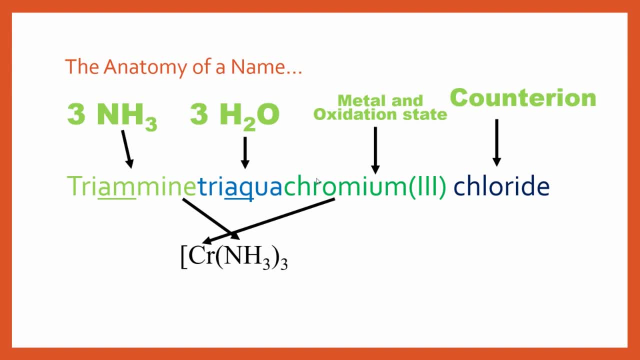 We look at the next bit. we've got triamine, so we're going to have NH3, which is amine, tells us that. and we've got the tri, telling us that we have three. Then we've got the triaqua, so there's your three H2Os, and then you've got the counter ion, and I'm just going to put that on the end. 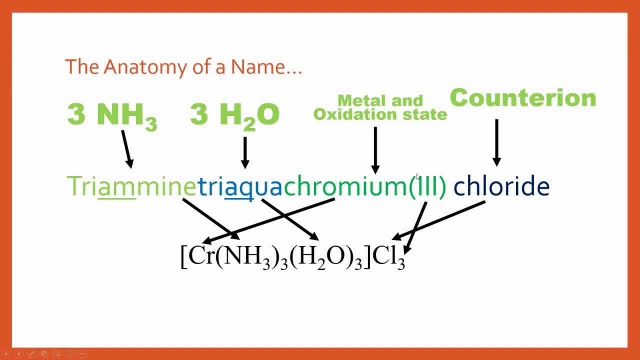 and because we know that we've got chromium and we've got that three there, we can figure out that it's got to be three chlorines in order to balance it out, to be overall Neutral in our coordination compound. so that is the anatomy of the name and by looking at this, 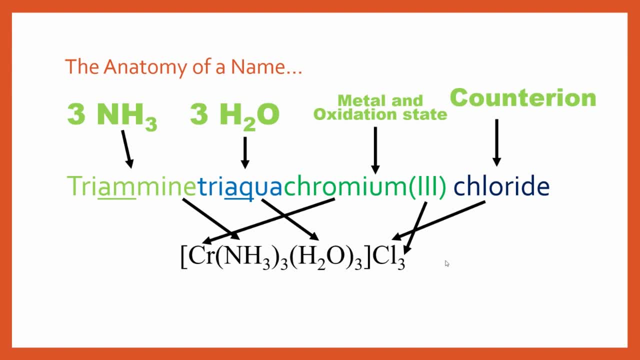 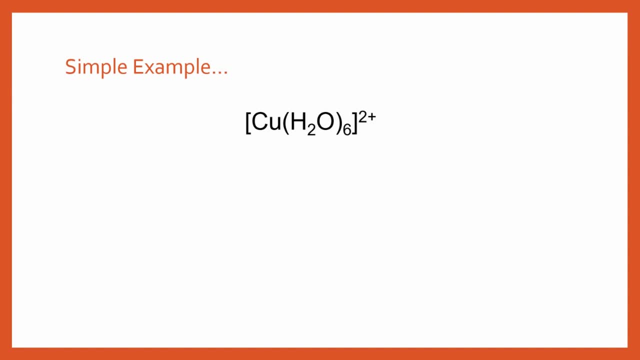 example and studying it. it's going to help you understand the work examples I'm just about to go through and, for the first example, I'm going to make it as easy as possible. I like to start with really simple examples to be really clear about how to do these, and then slowly build up to more. 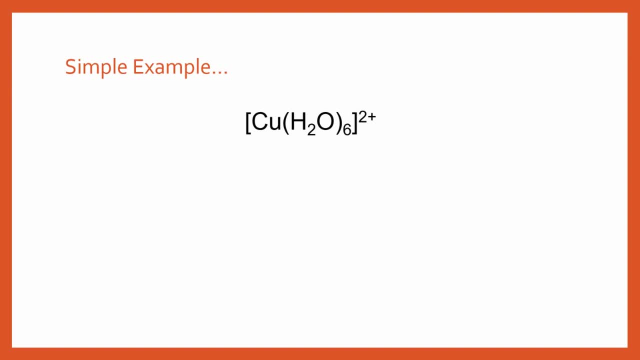 complicated examples, to focus on just one thing at a time. So here is a simple, complex ion and we are going to use what we've looked at before to break it down and work out a name. So the first thing you would notice is that this is a cat ion, so we've got a plus charge and you can remember. 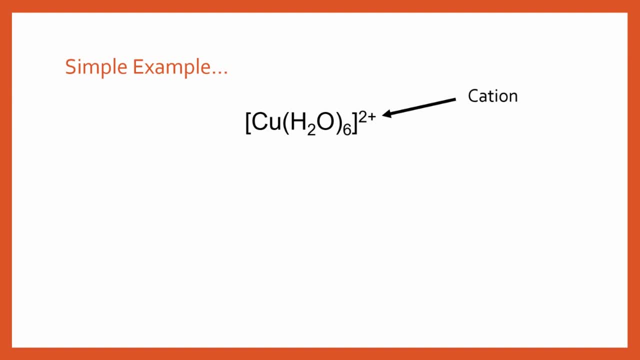 that another name for a cat is a pussy cat and cat ions are positive. so that's one way of terrible way of remembering that cat ions are positive. So we've got a positive charge there. that's going to be important in a second. So what we would first realize? we've got six of those, so that's going to. 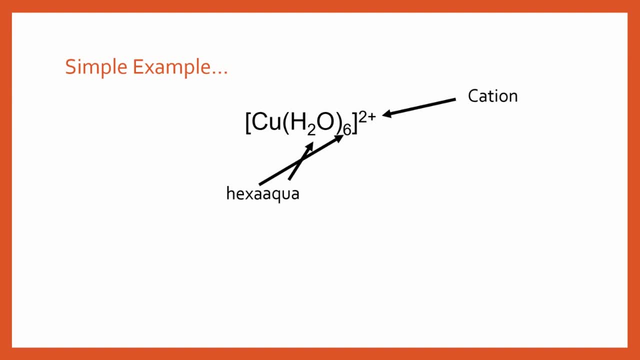 be an H2O ligand, so that's going to be aqua. and then we look at our table and I've cut from the table before. so we've got copper and if it's anionic it's going to be cuprate and if it's a, 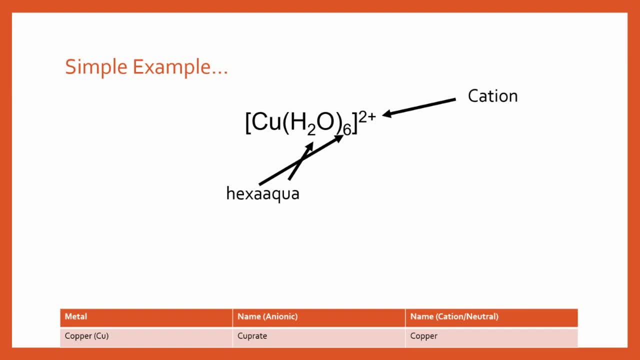 cat ion or neutral. it's going to be copper, and in this case we've got a cat ion, so that's going to be copper, and then we would need to work out the oxidation state of the copper, and so we'll realize that the H2O is going to be neutral. 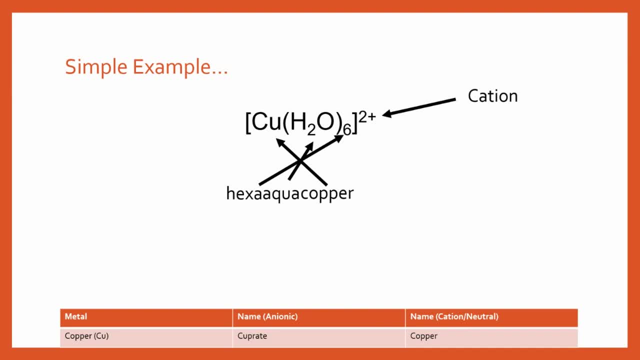 the copper is going to be our unknown, so we could call that x and all of that's going to add the two. so we could say x plus zero or six times zero, which is still zero, equals two. we solve for x- and I really hope that's not difficult- and we get x equals two. so what we can do is we can put a two. 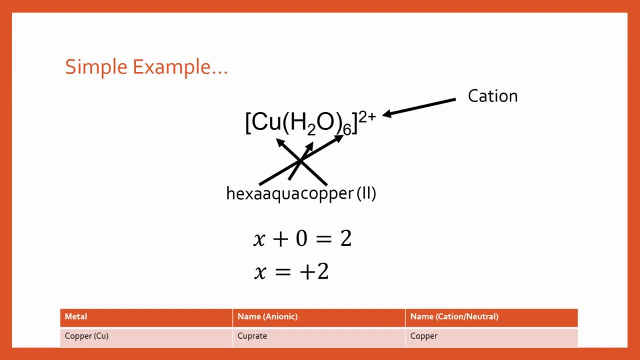 there and that's the name of this simple, complex ion. now, that's a very, very simple example. let's slowly move on to more complicated examples and introduce a little bit more of the naming. so let's look at this example. not wildly different. one difference is that, instead of having a two, 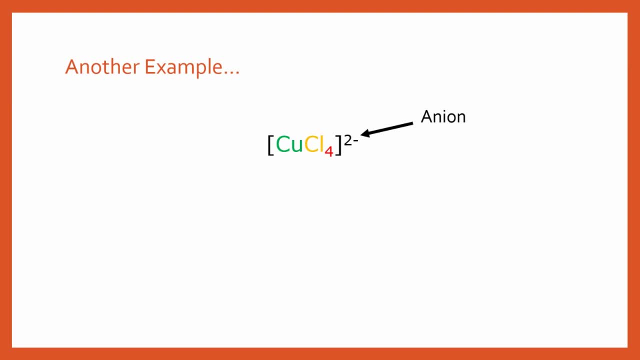 plus, we have two minus, so this is now an anion. so we're going to name it very slightly differently and I've color coded this to make life easy. so we've got that table there and that's going to be useful in a second. so we've got tetra and you see the red four, the red tetra. that's going to. 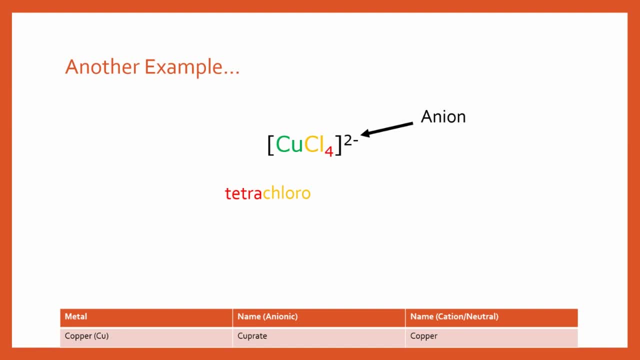 match up. then we've got chloro- and that's our name- that we would use for a chloro right ion or the ligand of chlorine. so we've got chloro there, and then we've got cuprate, and the reason we've chose cuprate is because we've got an anion. now we need to work out the oxidation. 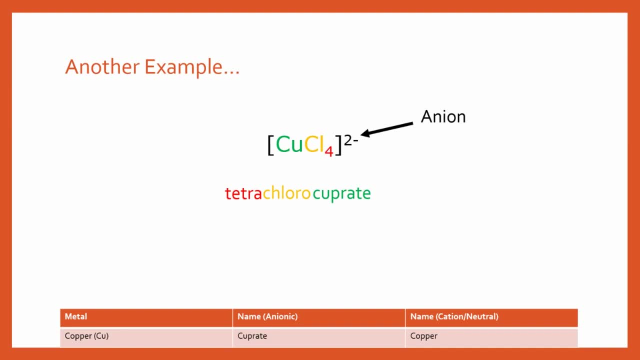 number and chlorine is going to be minus one, and so we've got that and it's all going to sum to minus two. so we get x for the copper plus four times minus one is minus two. simple algebra. you can solve that, and that means that x is going to be plus two. so we get a two plus four times minus. 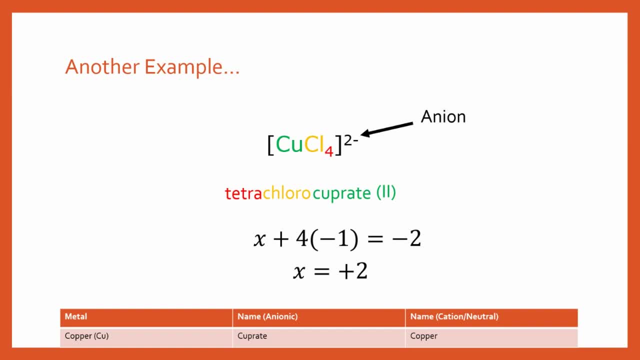 two there, and that's how you do this one. it's basically the same thing: we're just changing from a cation to an anion and getting a slightly different name. let's move on and look at another example, and this one I'm going to call an annoying example, and it's one where it's very easy to work. 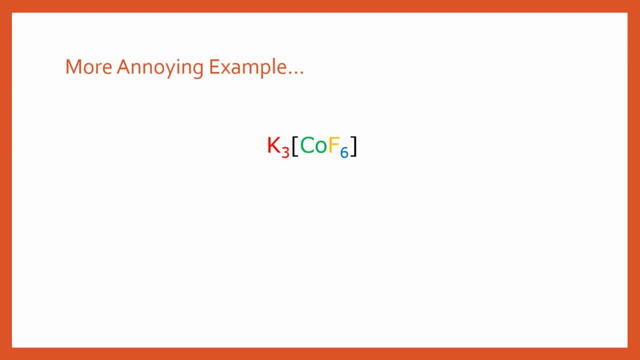 out the wrong name without realizing something. so we look at this and obviously potassium is going to form a positive ion. so I'm going to put a little plus beside that potassium just to help figure things out. so if you've got three pluses and overall this was going to be neutral, the bit with the cof6 outside the square brackets that's going. 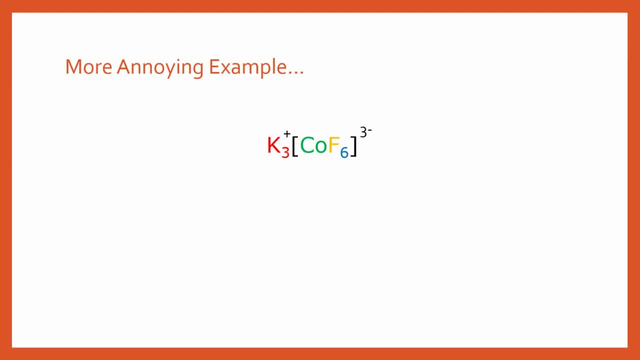 to have to be three minus. so we've got three pluses from the potassium, so we're going to have to have three minuses to balance that out. that is now important, and you'll see why in just a second. so we've got potassium at the start of the name. then we're going to have hexa for the six f and 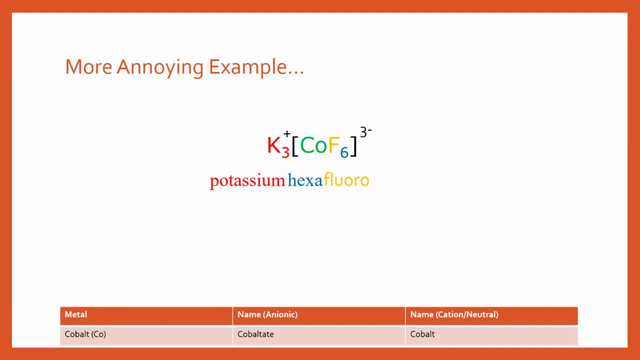 then fluoro, and then we look at the list here. now we've got to decide if it's going to be cobaltate or cobalt, and we can see that we've got that three minus there. so we're going to choose cobaltate. now what? 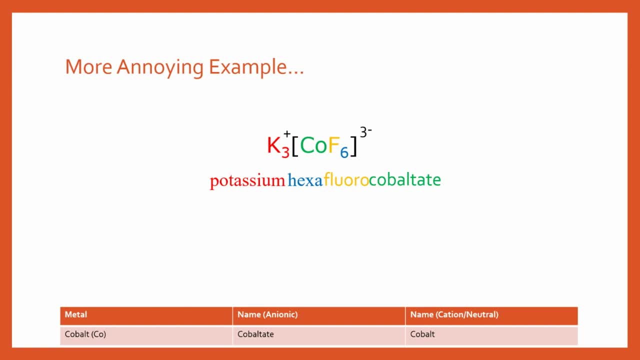 we need to do is you can realize that overall this is all going to sum to zero. so we could say that we've got cobalt plus three potassiums plus six fluorines, and this is just a kind of place holder for the oxidation states. so replace the symbols with the oxidation states. so cobalt's 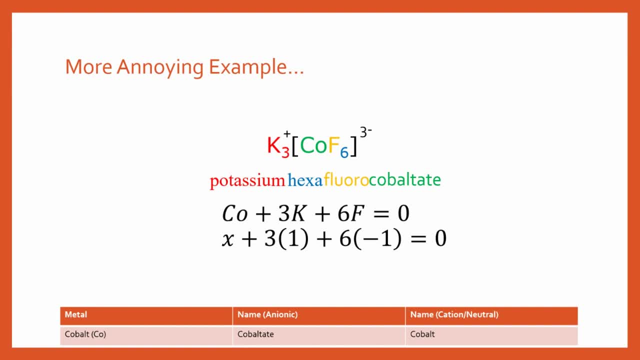 going to be x? that's our unknown. the potassium is just going to be plus one and the fluorine is going to be minus one. we know that's all going to sum to zero. and then you can simply solve for the oxidation state of cobalt, which is three, very, very simple algebra, and so 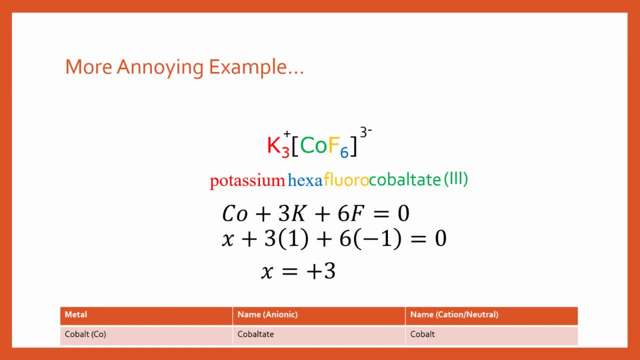 that lets us put a three on the end of there, and that's us worked out this name. don't be caught out. many people would just call this cobalt, which is incorrect. it should be cobaltate and that's how you do that one. the next thing i want to talk about is some situations where you would have